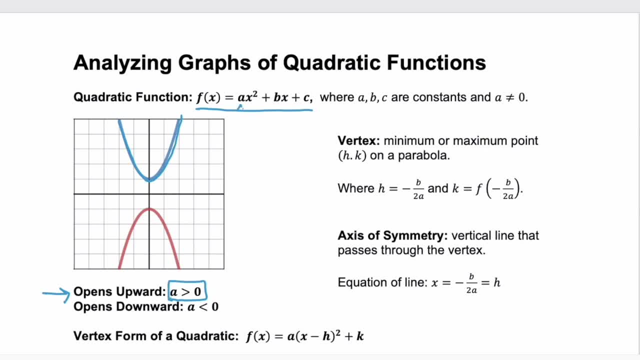 the a value that leading coefficient is greater than zero, It's not a negative number. When we have a negative number, we have a negative number, So we have a negative number. It will open downward and we'll have a graph that looks similar to this red quadratic. 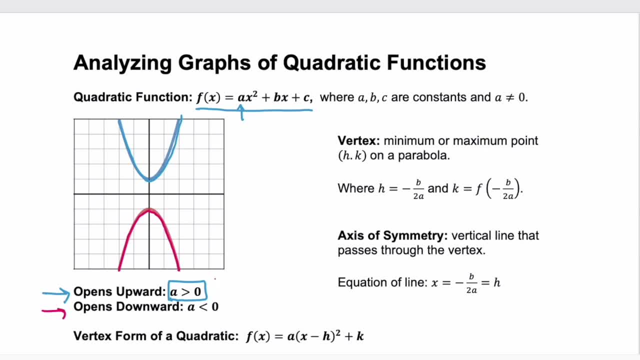 That's a very important key because it helps us figure out if we're going to have a minimum or a maximum, And a minimum or a maximum refers to our vertex. Vertex here is going to be this point h, k, And I know the letters are a little bit different than what you've probably seen. 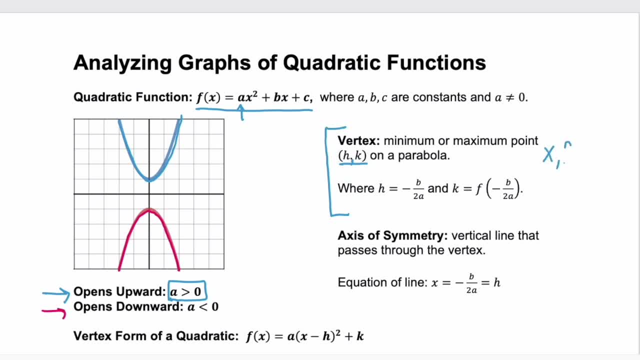 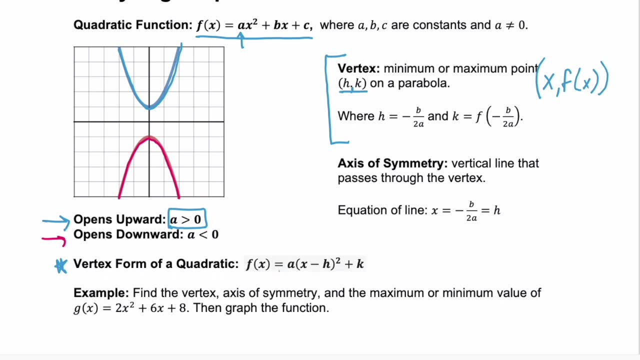 before. You may have seen x and f notation before. Same thing. they're only using h and k in this book because if you look down here a little bit further on the page vertex form of a quadratic, If you're given that h and k, the vertex, you can find the equation for 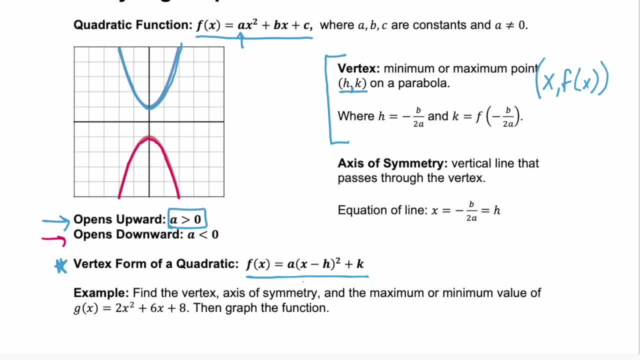 the quadratic using this form, But again it's still. it's an x value and it's a y value. You find that x value or h here, the exact same way. It's negative b over 2a where the b and the a refer to the a and the b in our quadratic function of ax squared plus bx plus c. 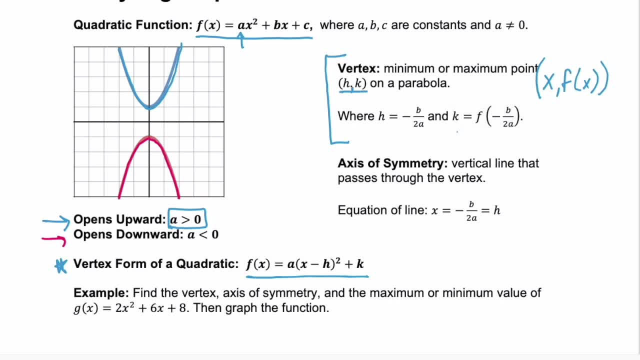 And then you find your k or your y value by plugging that x value back into your function, So that vertex, remember, tells us if we have a minimum or a maximum, And the x value or h- here is our axis of symmetry. 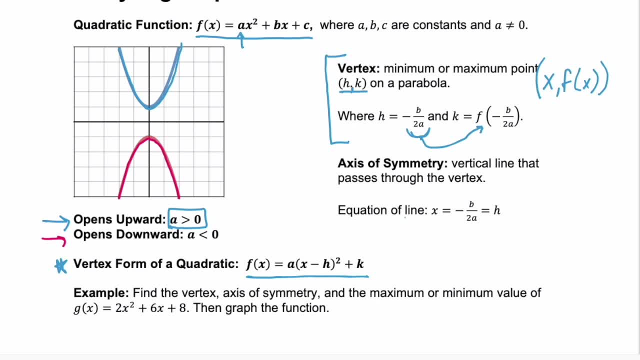 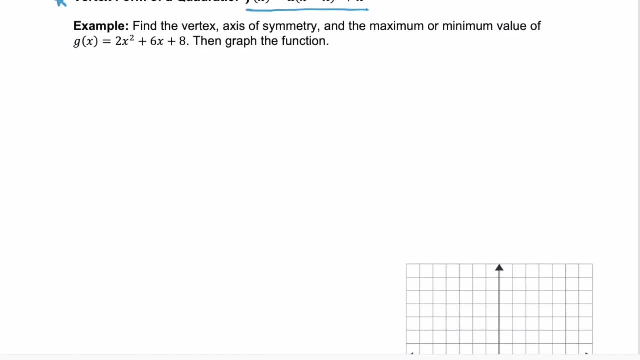 Remember, the axis of symmetry is a vertical line that cuts that parabola perfectly in half And it's in the format: x equals negative b over 2a. Enough explanation, Let's look at. Let's look at our first example. 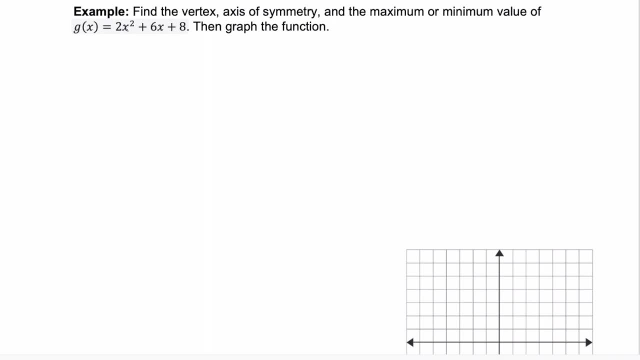 We're given a function: 2x squared plus 6x plus 8.. And we need to find the vertex, the axis of symmetry and the maximum or minimum value of g of x, And then we need to graph the function. 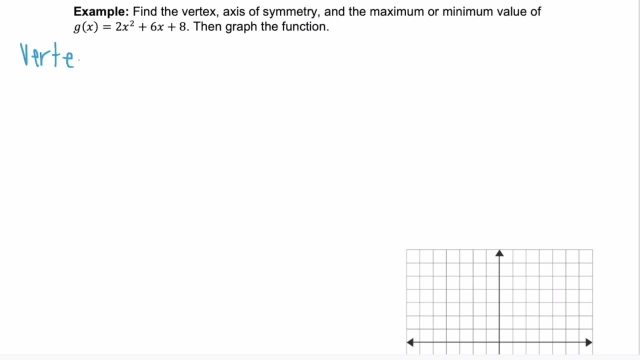 So start with our vertex. Remember that the x or the h value here is equal to negative b over 2a, Our b is 6 and our a is 2.. So this simplifies to negative 6 over 4 or negative 3 over 2.. 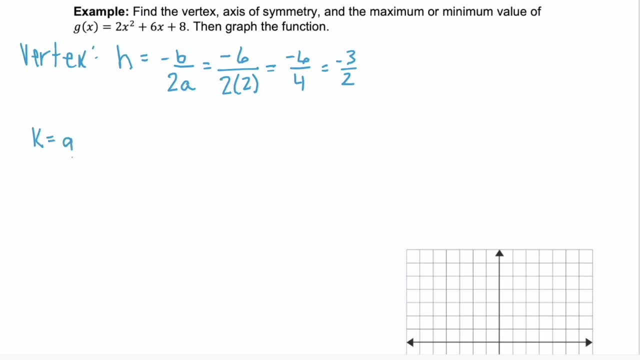 Then to find k, we are just going to solve g of negative 3 halves. So we're substituting in this x value we just found into that given function. So 2 times Negative 3 halves squared plus 6 times negative 3 halves plus 8.. 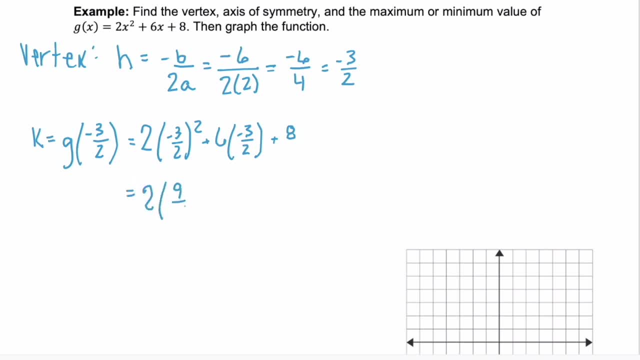 If we square the negative 3 halves, we get 9 fourths Plus 6 times negative 3 halves is negative 18 halves plus 8.. Let's simplify a little bit more: 2 times 9 fourths, 9 fourths is 9 halves, because the 2 and the 4 simplify to just the 2 in the denominator. 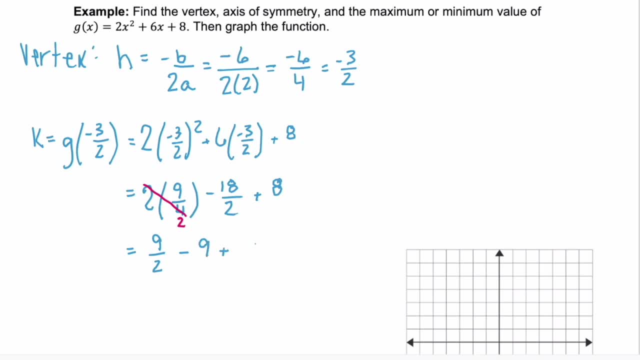 Negative 18 halves is negative 9, plus an 8. Add all of these values together and we'll get 7 halves. So our vertex- Remember, vertex is a point, So it needs to be an ordered pair notation. Our vertex here has an x value of negative 3 halves and a y value of 7 halves. 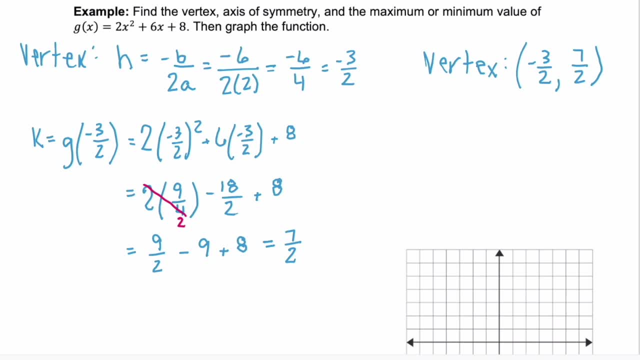 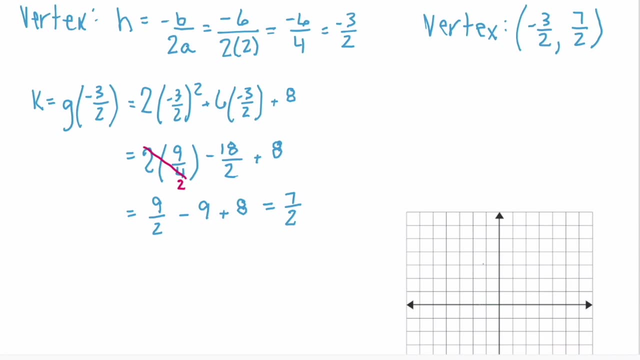 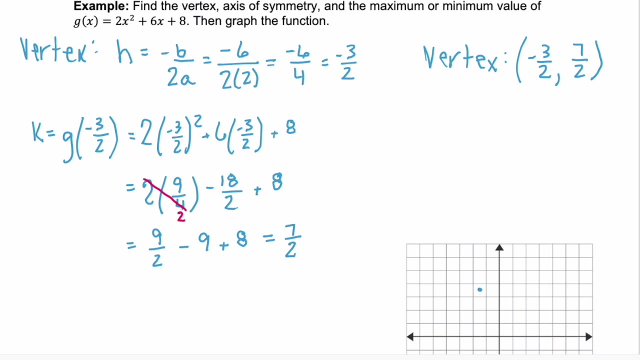 We can graph that right away on our graph here. So negative 3 halves is negative 1 and a half, And 7 halves is 3 and a half. So our vertex is this point Now do we have a minimum or a maximum? 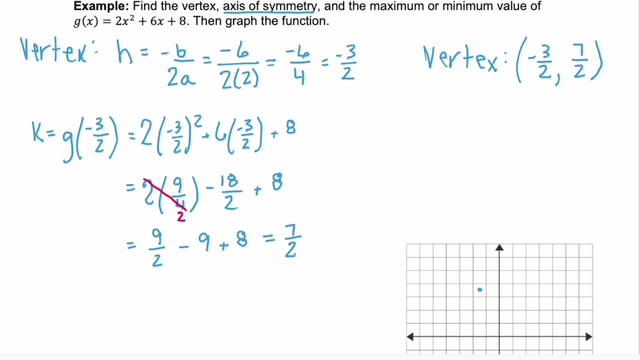 Oh wait, hang on. Axis of 7. Symmetry: Remember your axis of symmetry. That is x equals and it's the x value of your vertex. So our axis of symmetry is the equation: x equals negative 3 halves. 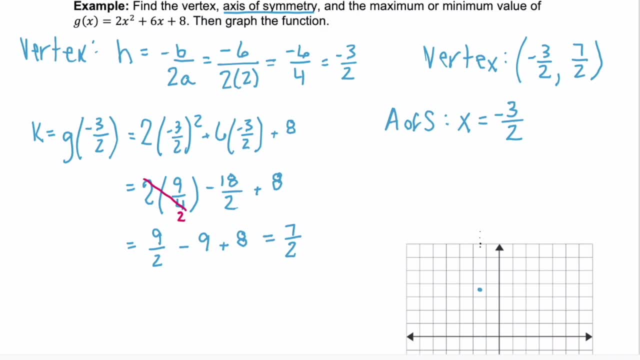 So I'll do a dotted line here. It's this vertical line that goes right through our vertex. Okay, Do we have a minimum Maximum or a minimum? Well, let's go back to our function. g of x equals 2x squared plus 6x plus 8.. 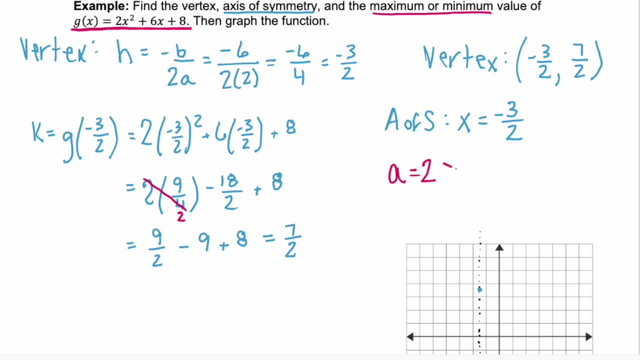 Our a here is equal to 2.. 2 is greater than 0.. So that tells us that our graph opens up Or we're going to have a parabola that looks like this: If we have a parabola that opens up, our vertex is going to be our minimum. 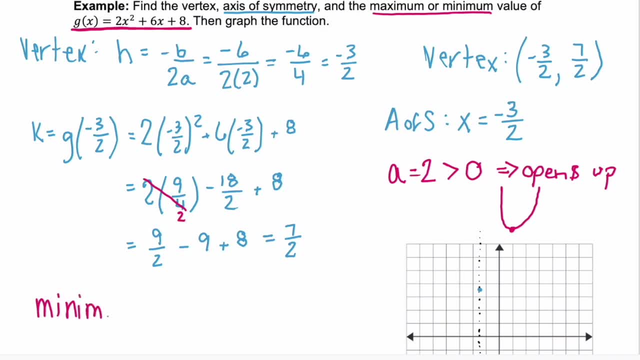 So we're going to have a minimum value. When you're asked for the minimum value of a function, It wants to know the lowest y value And the lowest y value you'll have is going to be the y value of your vertex. So your minimum. 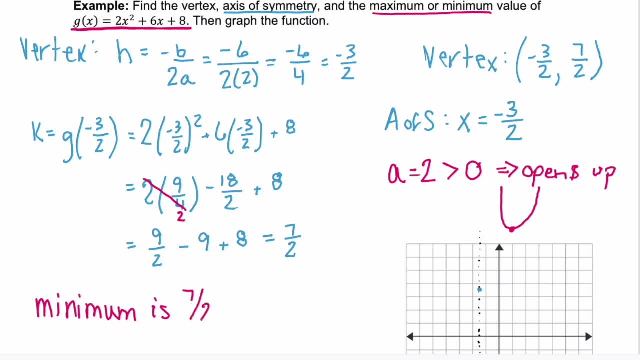 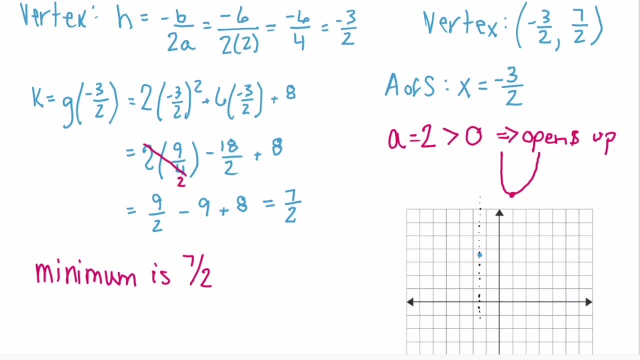 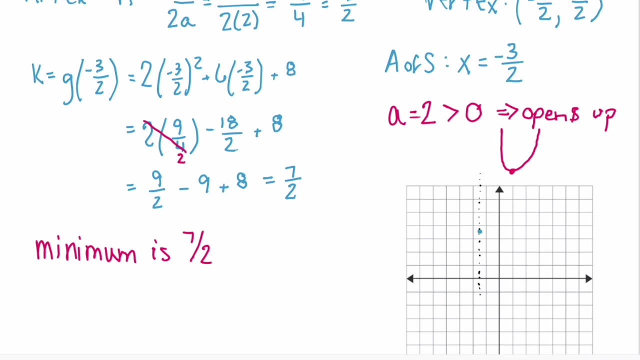 is 7 halves. Now we need to finish our graph here, and to do that we want to find at least two more points, and technically we can find just one more point and use our axis of symmetry as a mirror to give us that third point, The. 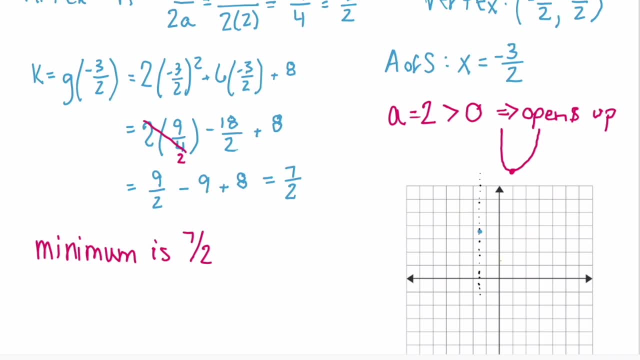 easiest point for us is going to be able to find our y-intercept. So our y- intercept is when x equals 0. So we need to solve 2 of 0 squared plus 6 times 0 plus 8, and that's 0 plus 0 plus 8. 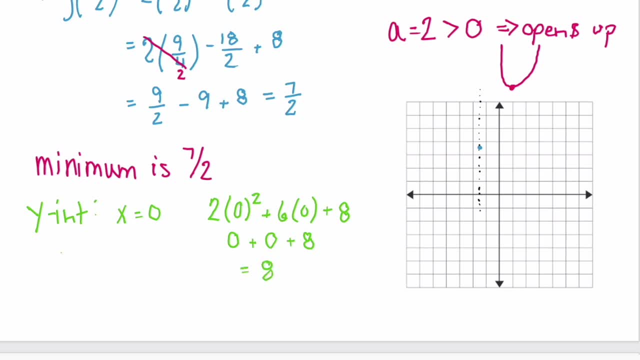 or 8.. So the y-intercept is this: point 0, 8.. If we plot that, that would be up here The mirror image of this. So this point is one and a half squares from our axis of symmetry and it's one and a half squares to the right, So it has a mirror. 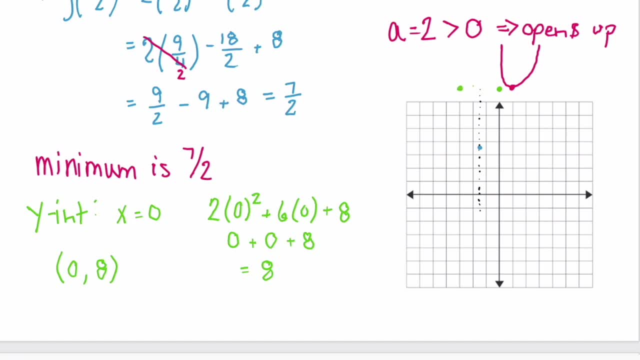 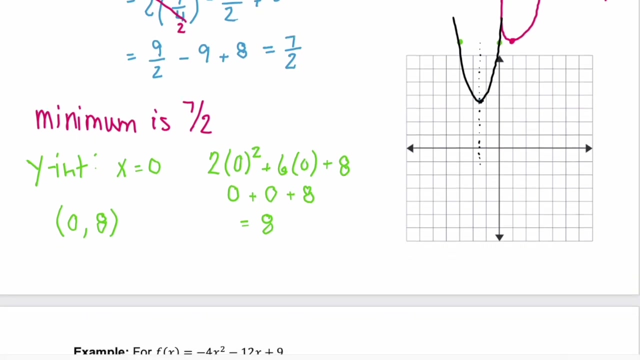 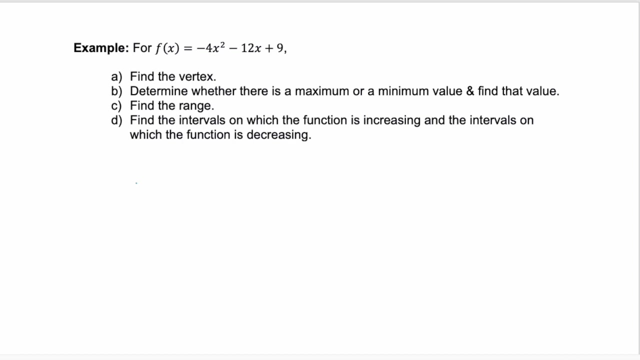 image one and a half squares to the left. Then if we connect those dots we get the graph of this g of x function. For this example of analyzing a quadratic function, we have four different parts to solve. Part a: we need to find the vertex and we're pretty comfortable. 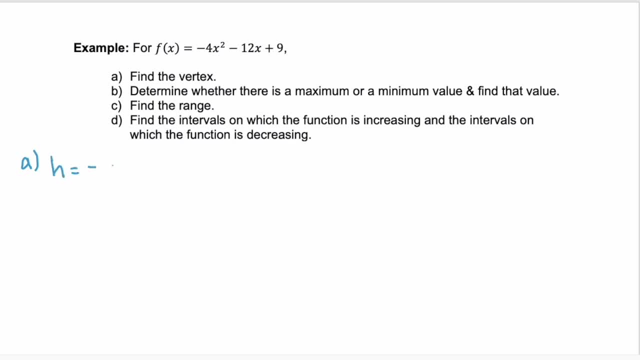 with that, The h value or the x coordinate is negative b over 2a. So we have a negative and b is negative 12.. So negative negative 12 over 2 times a, which is negative 4. That becomes 12 over negative 8, which simplifies to negative 3 halves. 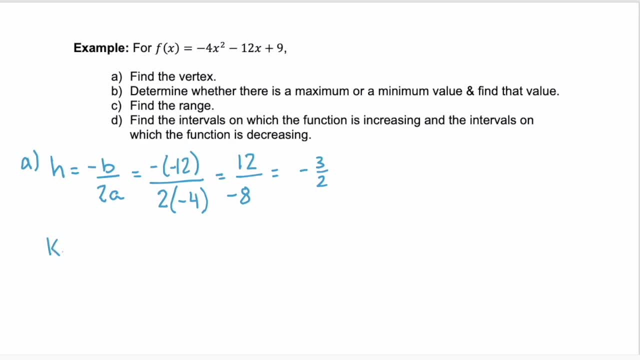 Then, in order to find k, we're going to solve f of negative 3 halves. So we substitute in the negative 3 halves wherever we have an x. So negative 4 times negative 3 halves squared minus 12, times negative 3 halves plus 9.. 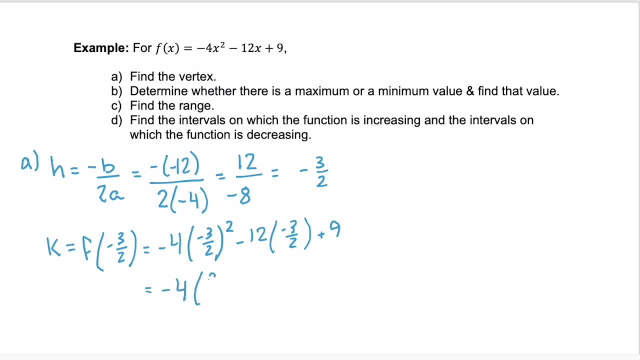 Simplify the negative 3 halves squared. That becomes Here: we have a plus 36 over 2, plus 9.. Negative 4,, which is negative 4 over 1, times 9 over 4.. That simplifies to negative 9, right. 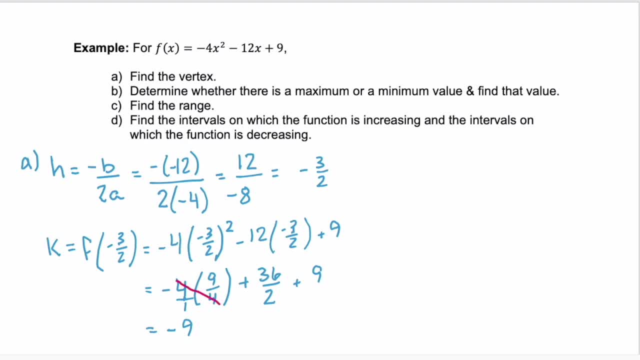 Because these 4 simplify out as 1.. Plus 36 over 2, which is 18.. Plus Plus 9.. The 9s are going to cancel each other out, so we're left with 18.. So our vertex is going to be the point negative: 3 halves 18.. 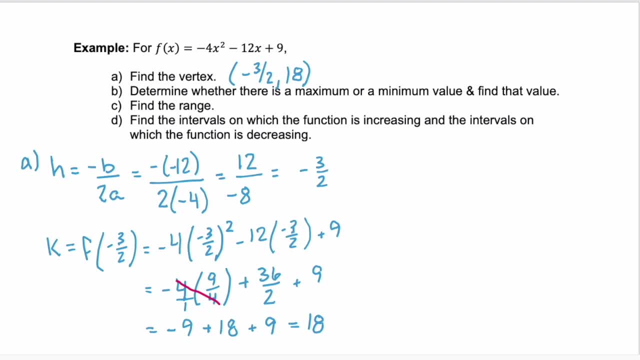 Now we need to determine whether this is a maximum or a minimum, And then we need to find the value. Well, we know the value is going to be 18.. But we need to know: do we have a maximum, or Do we have a maximum or a minimum? 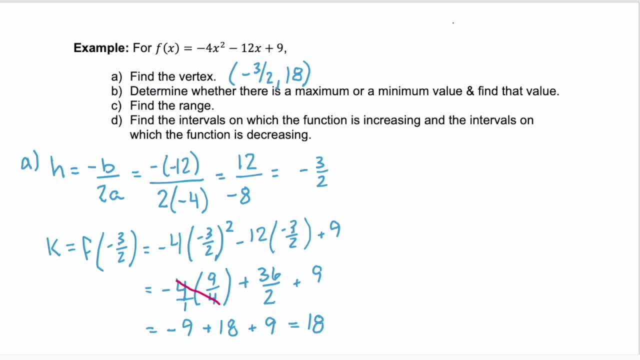 And to do that, we need to know what a is. Well, our a value is equal to negative 4.. That tells us that our graph will open down, And if it opens down, it looks like this: right, That means we have a maximum. 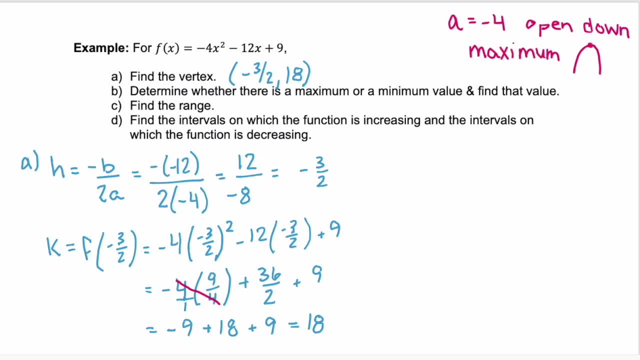 Our vertex is going to be the highest point, So we're going to have a maximum. And remember, the maximum or minimum value is always the y-coordinate of your vertex, Because that's the tallest or the highest y-value that your graph ever has. 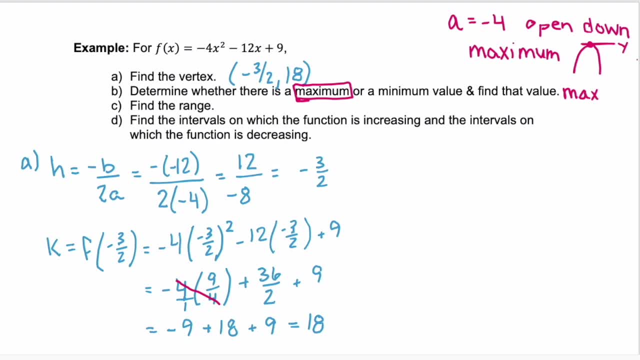 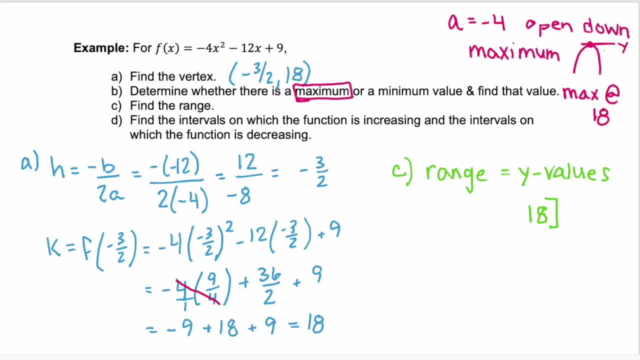 value. We put a bracket at 18 because we get to the point 18, that's our vertex, and our y values can get smaller. right, The graph is going down, so it's going towards negative infinity for the y's, So our range is negative infinity through. 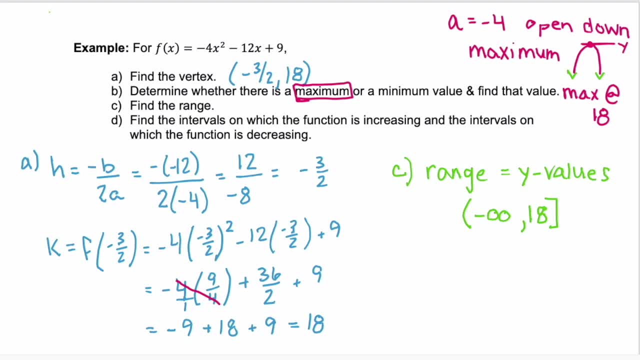 18.. And part D wants to know the intervals on which the function is increasing and decreasing. So increasing is our first interval, right, Because our graph is going towards that vertex, towards the maximum And the intervals that it's increasing. that's the possible x values. Well, it's increasing from. 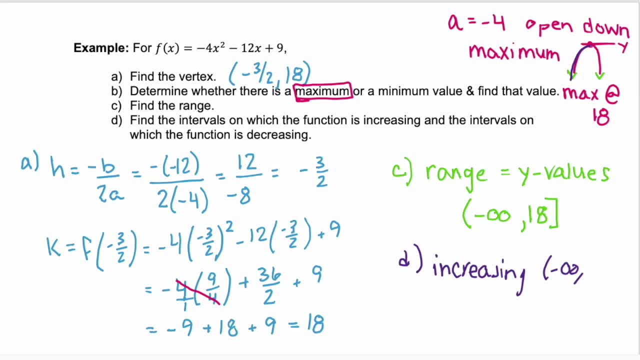 negative infinity until it gets to that vertex. And what value is the x value of our vertex? It's negative 3 halves. So from negative infinity to negative 3 halves, for x our graph is increasing And then it's going to be decreasing on the other half, So it starts to decrease at the vertex of. 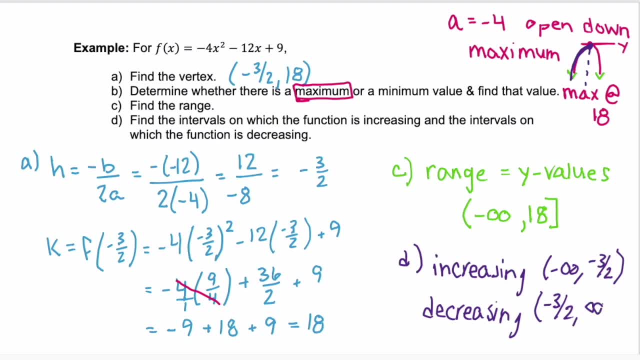 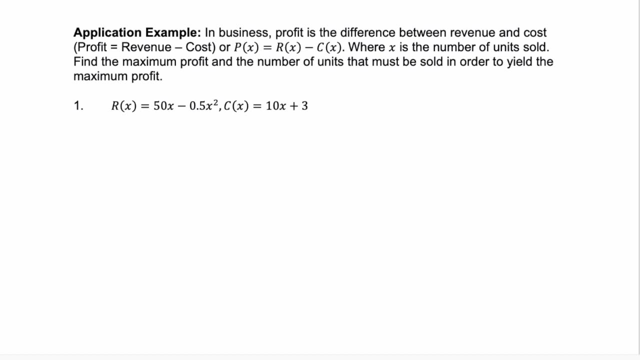 negative 3 halves and continues to decrease through positive infinity. One last problem, and it's an application problem: It's all about the number of y's. So we're going to calculate the profit function for a business. Remember that profit is equal to revenue minus. 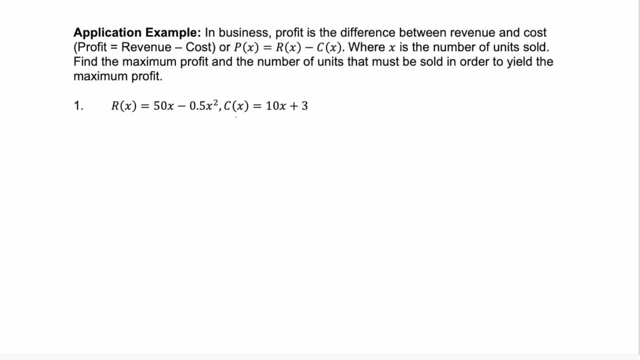 cost and we're given the revenue function and the cost function. So to find the profit function we need to subtract those two. So we take the revenue function and we subtract the cost function. We want to put that cost function in parentheses because our next step is to distribute that. 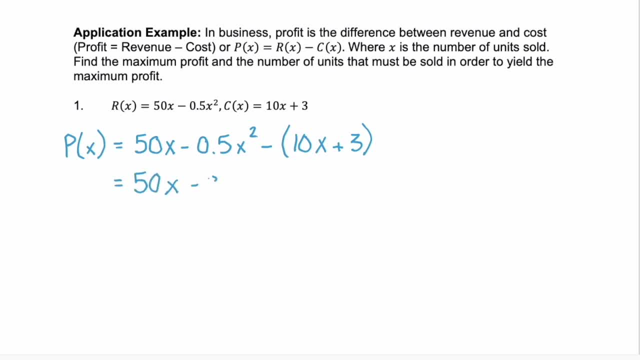 minus sign. So we have 50x minus 0.5 x squared, minus 10x minus 3.. Now let's rewrite it into standard form. So we want our x squared term first, That's a negative 0.5 x squared. Then we have plus. 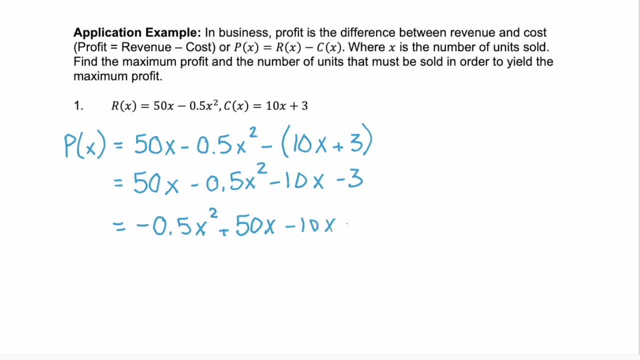 minus 10x minus 3.. We can combine these two middle terms and that simplifies to negative: 0.5 x squared plus 40x minus 3.. So we have that profit function. Now we want to find the maximum profit. Well, remember the key maximum. 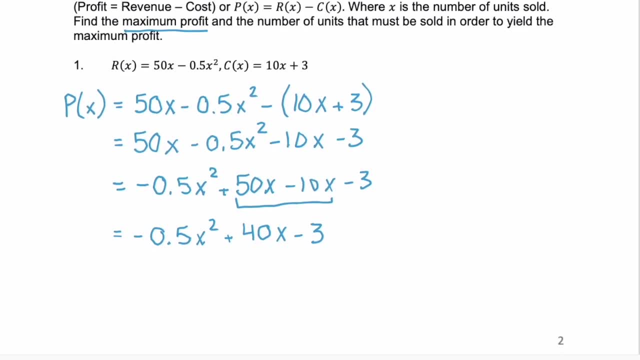 tells us that we need to find the vertex. So let's find that vertex and the h or the x value of our vertex is negative. b over 2 times a, which is negative. 40 over 2 times negative 0.5, which is negative. 40 over negative 1.